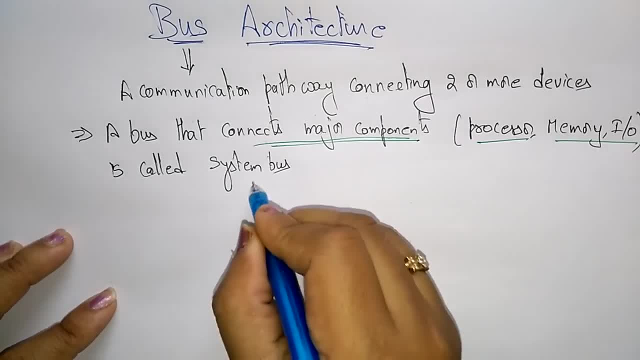 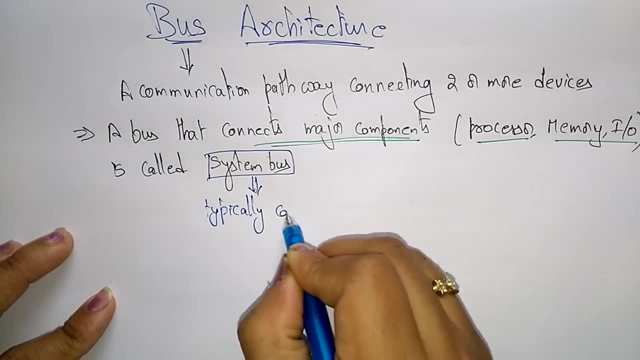 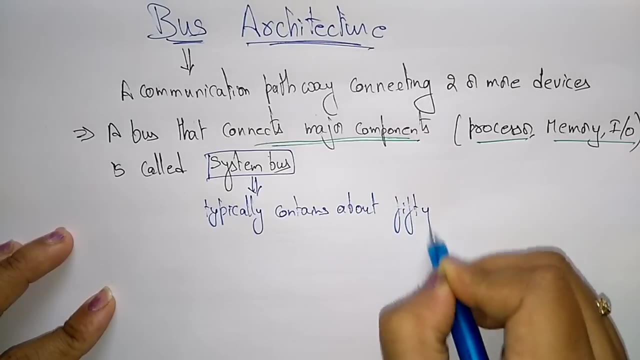 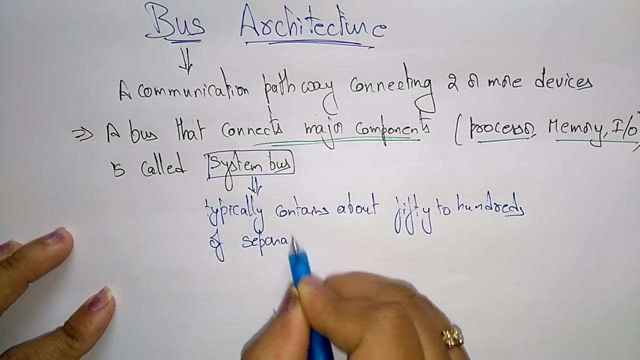 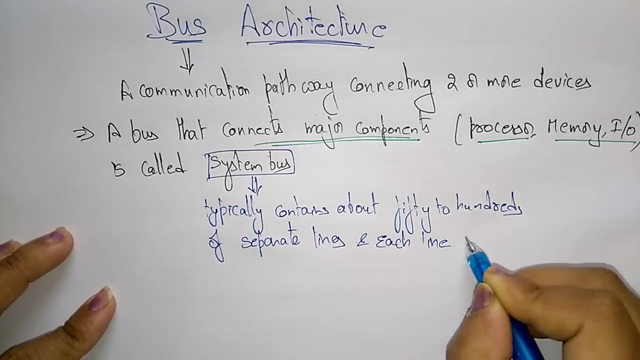 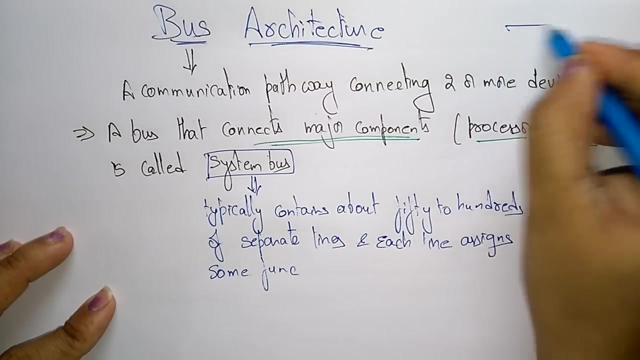 Actually, the system bus, whatever here it is, it typically contains this system bus typically contains about 50 to 100, 50 to 100 of separate lines, and each line assigns some function. What it means, Actually, whatever the bus you are taking, a bus consisting of set of lines. 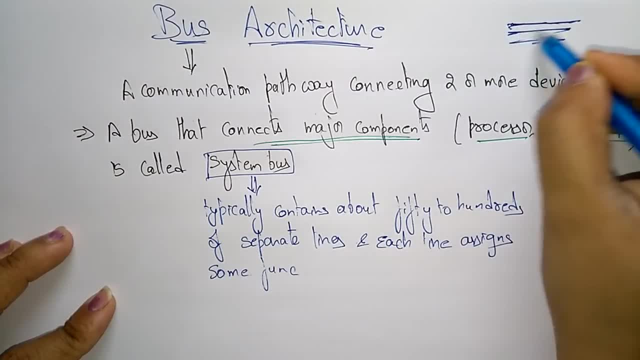 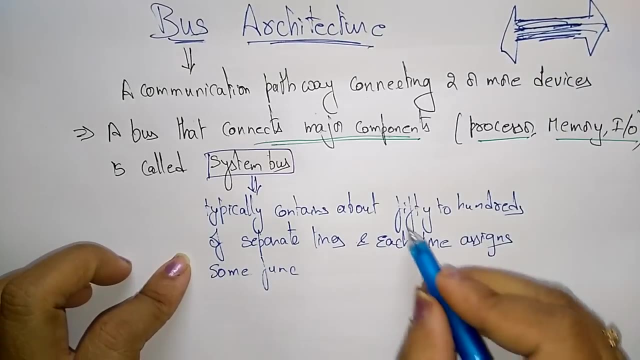 A single line. you call it as a bus. So a system bus consisting of set of lines will be there. Set of bus lines will be there. So these bus lines, this set of bus lines, may be 50 to 100. It is nearly 50 to 100- or present in system bus. 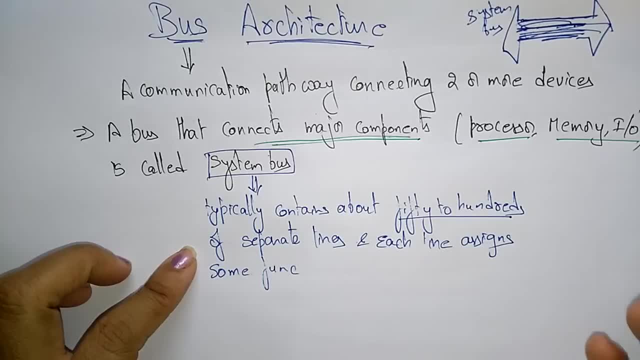 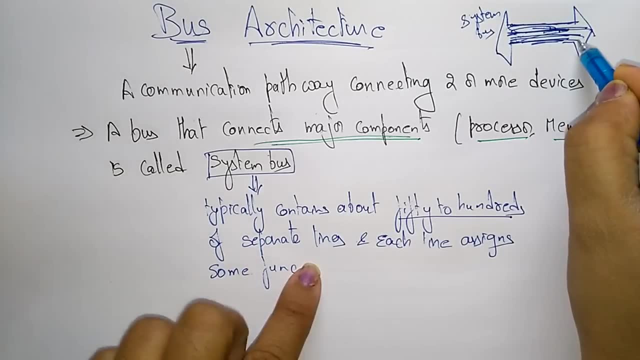 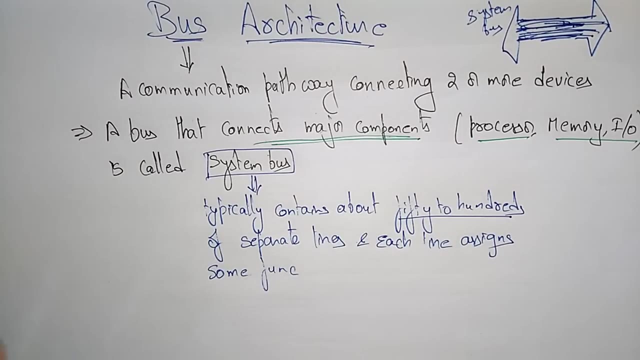 A system bus consisting of set of bus lines. Those may be around to 50 to 100. So each bus consisting of line line, so whatever the line, each line assigns some functions, means it is having some meaning. so that is a system bus, actually a system bus, usually separated into three functional groups. 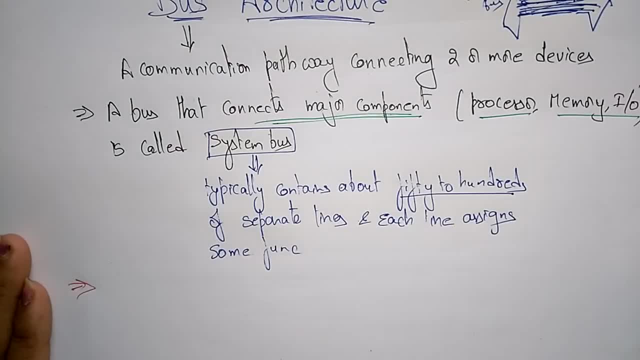 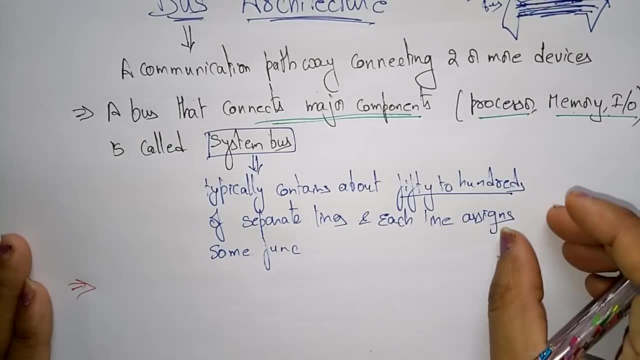 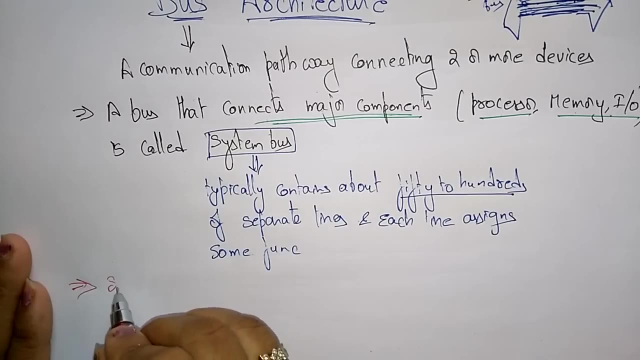 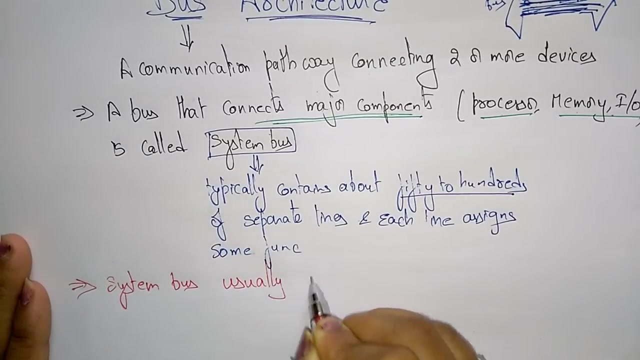 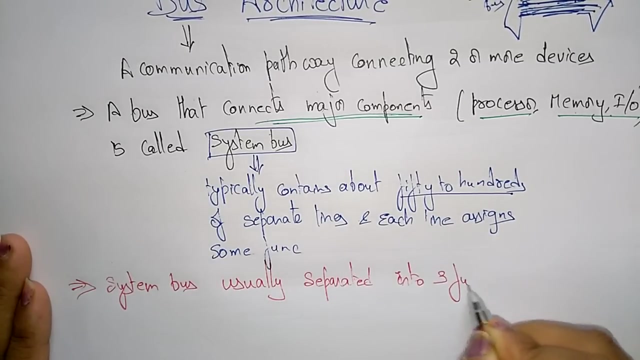 so, whatever the system bus means, it's just a communication it connector between these components- major components, processor, memory and ibook. and this system bus separated into three functional groups means the group of lines are separated into three functional groups. system bus usually separated into three functional groups. 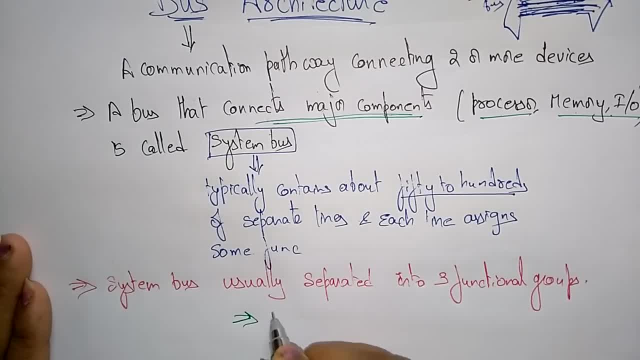 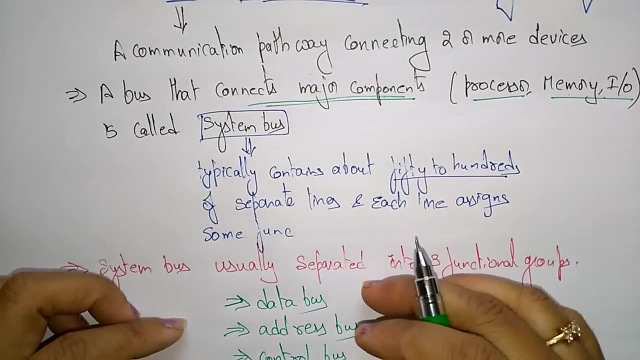 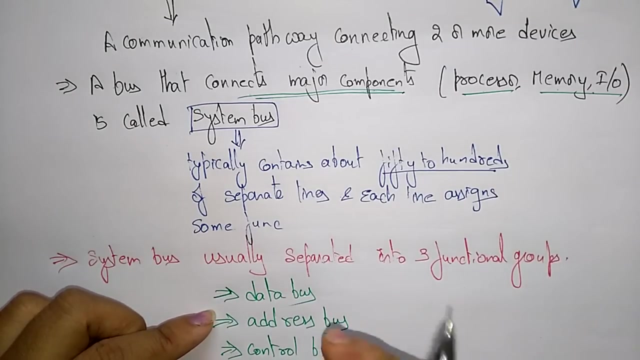 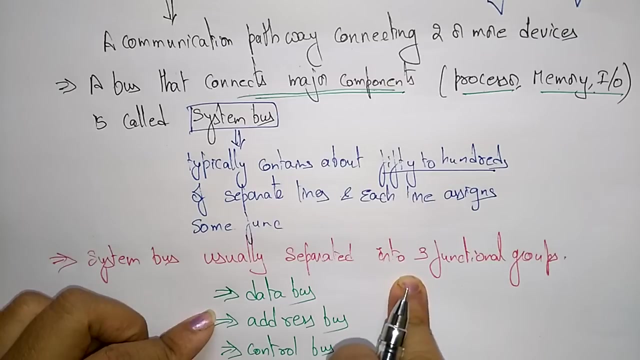 so those are data bus, address bus and control bus. so a system bus means a set of bus lines is divided into three separate buses: data bus, address bus, control bus. data bus is used to hold the data, whatever the data that processor has to work on and the processor is going to be stored, sent to memory and i5 devices and the 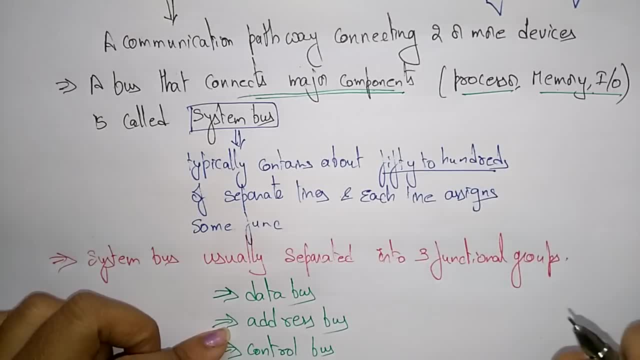 address bus is going to be stored in. the system bus indicates from where we have to get the data and from where we have to put the data. so that indicates the address bus. and the control bus is used to monitor the data and address, so it always monitors the system. okay, so these are the three buses. this call it as a system bus. 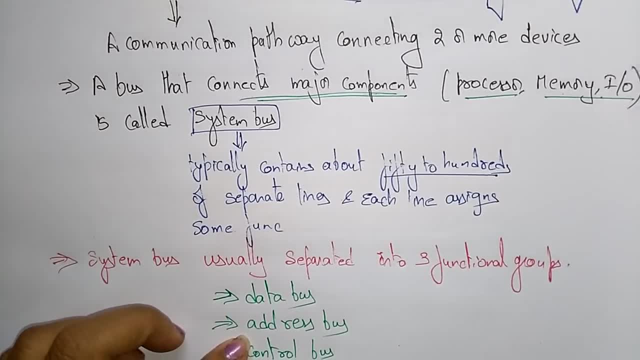 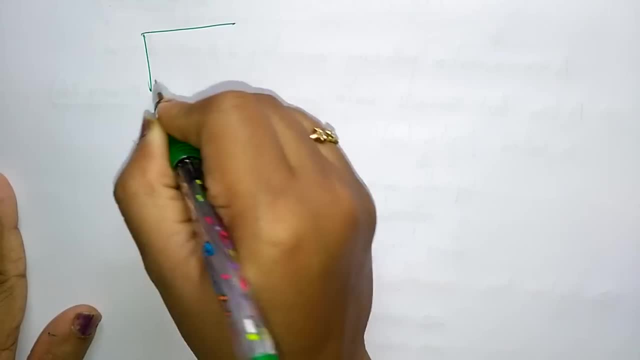 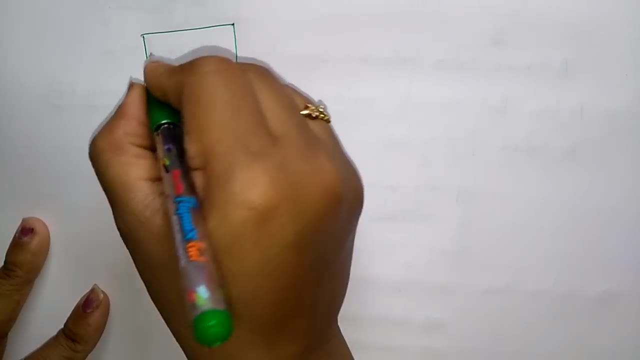 a system bus consisting of data bus, address bus and control bus. so let me explain this system bus with the diagram. so here i said the system bus is used to connect the major components in the computer system. what are the major components? cpu- the cpu consists of alu, arithmetic. 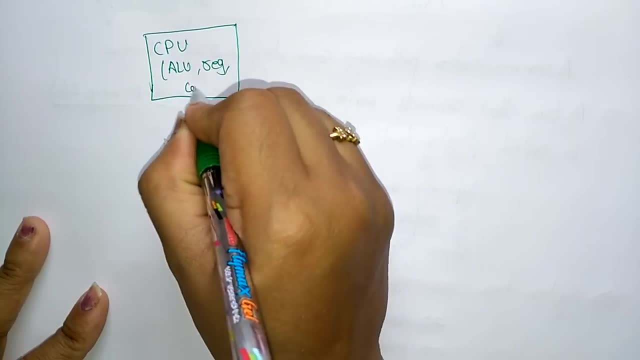 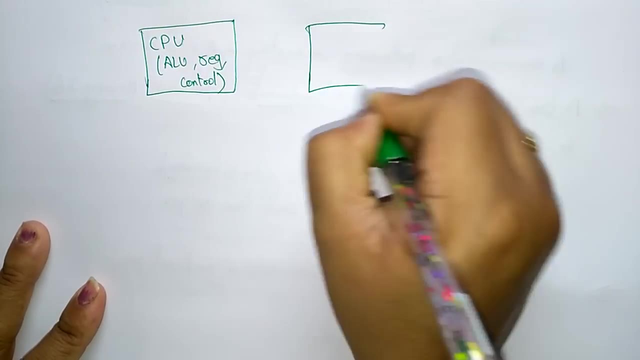 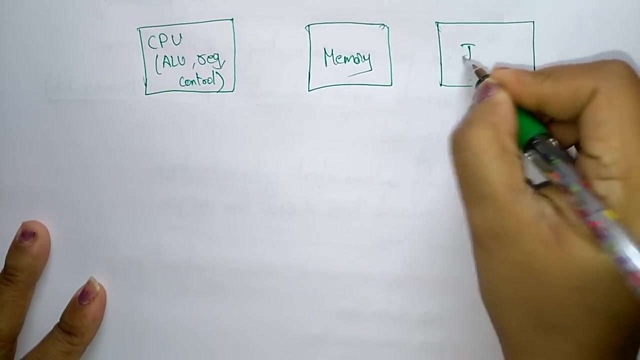 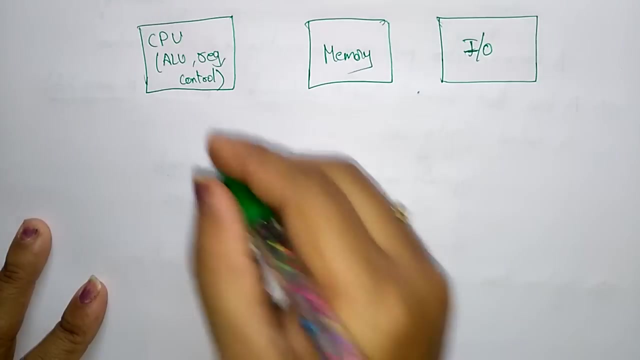 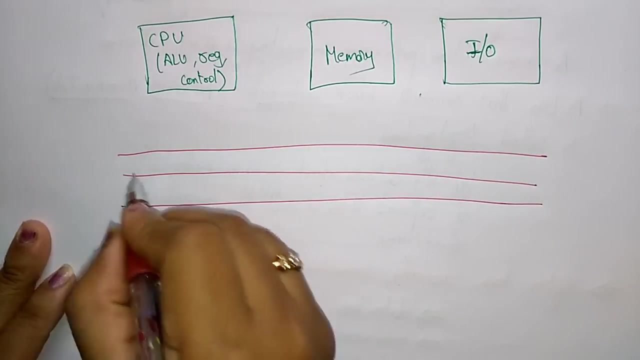 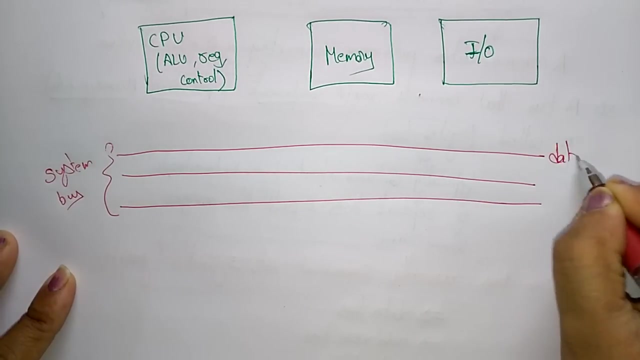 logic unit, registers and control unit. so this is one component: cpu memory, cpu, cpu- input output unit. okay, so these are the three major units. so these three major units are connected with the help of system bus. so this is a system bus. a system bus is having data bus. 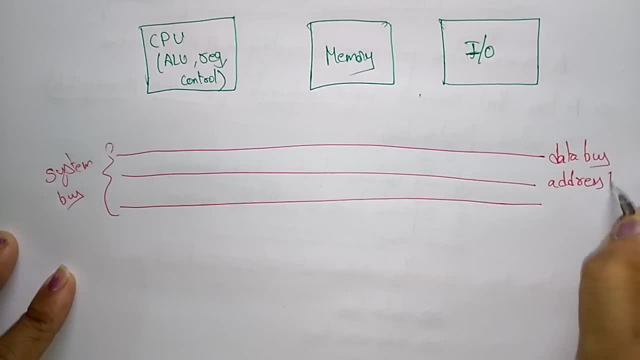 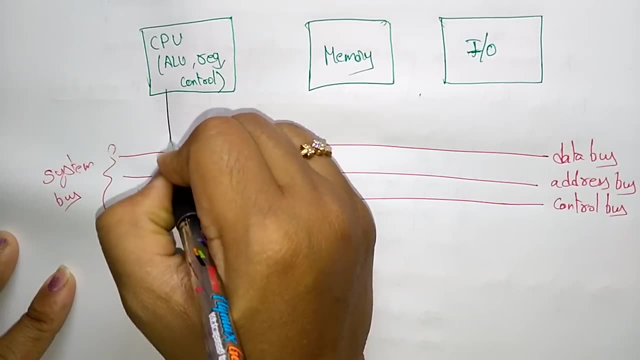 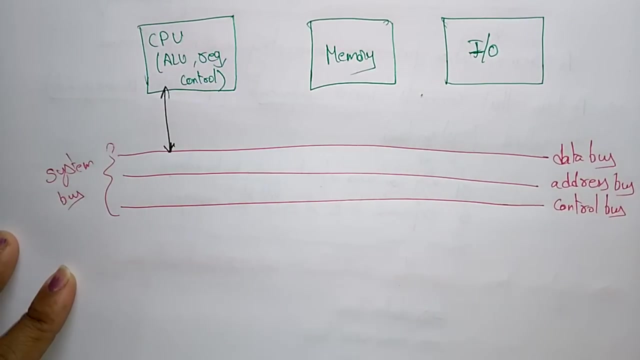 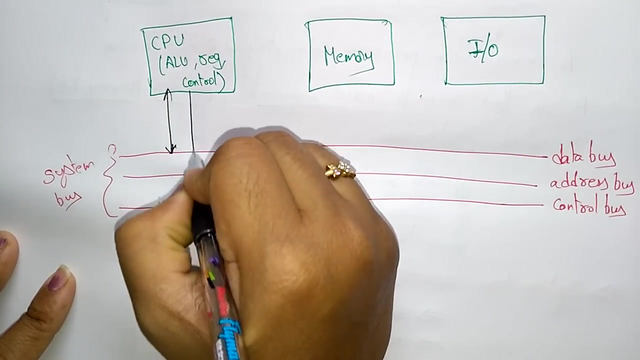 address bus and control bus Ç. so this system bus is connected to cpu. okay, so this is a data bus. a data bus is a bidirectional: the data is sent from other devices to memory and from in cpu to other devices, from other devices to cpu, and address bus is a unidirectional, whereas control bus is. 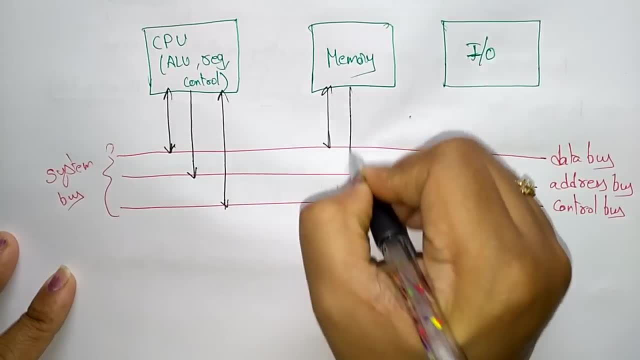 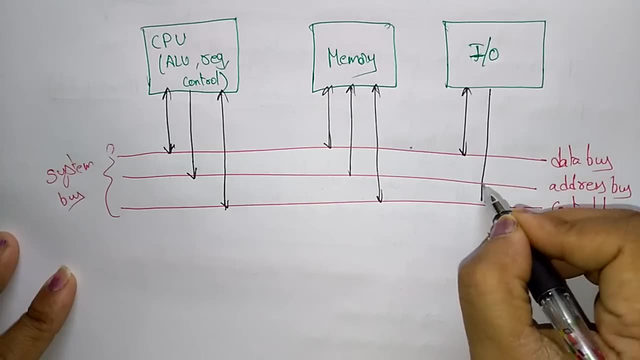 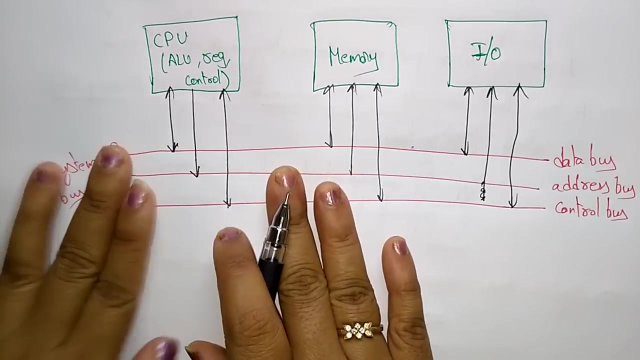 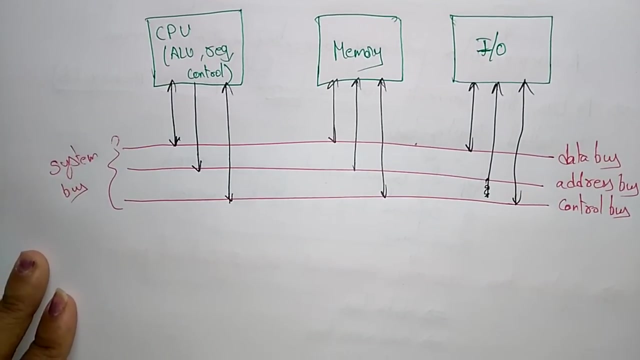 it's a bi-directional, in the same way for memory. okay, so this is a system bus, a system bus that are connected to a major components. let us discuss one by one. so first is data bus. so what is the use of the data bus in the system? 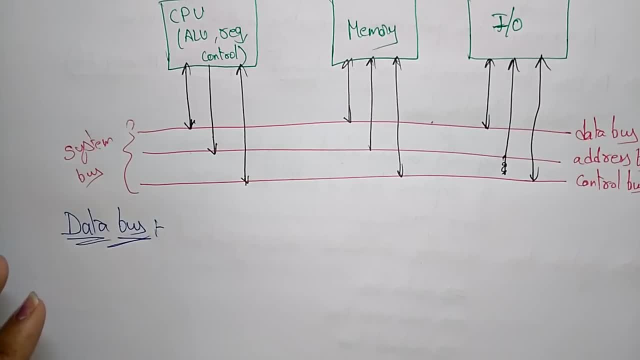 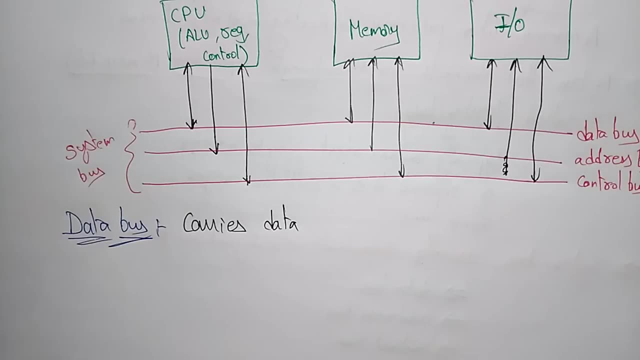 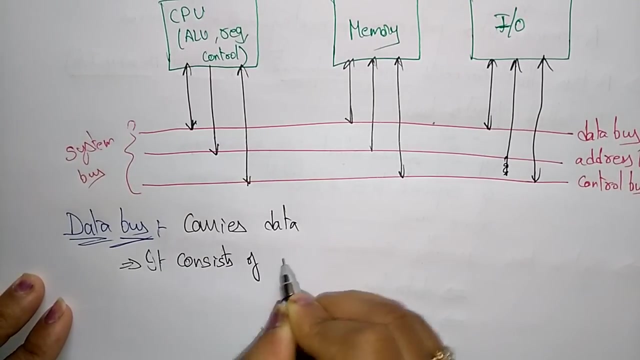 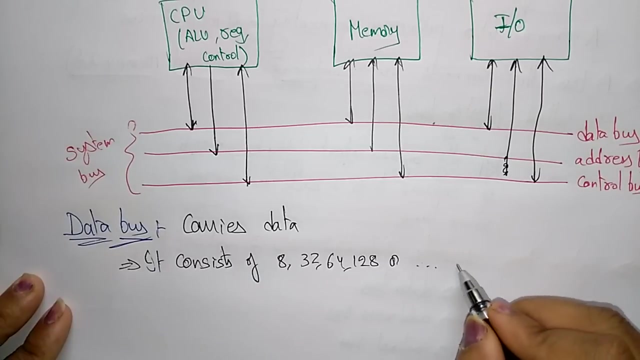 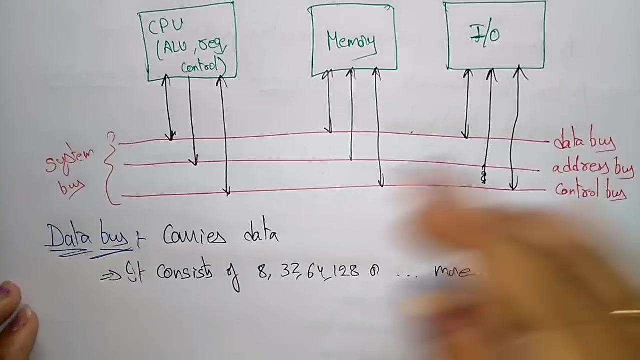 so a data bus is nothing, but it is used to carries data. it carries data from one device to another device. so it consists of: it consists of 8, 32, 64, 128 or, even so, on more separate lines. so again, this data bus is having separate lines. so I said, the system bus is nothing, but it is. 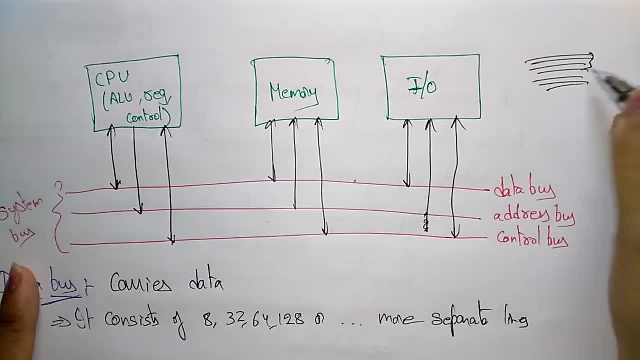 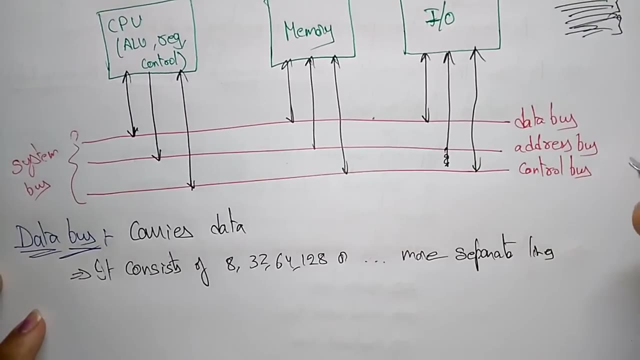 a group of lines. this group of lines is divided into data bus, address bus and control bus. so again, this data bus is having some separate lines, so those lines will be of size 8, 13, 64, 128 or it may be so on. so the number of lines here in the data bus, the number of lines. 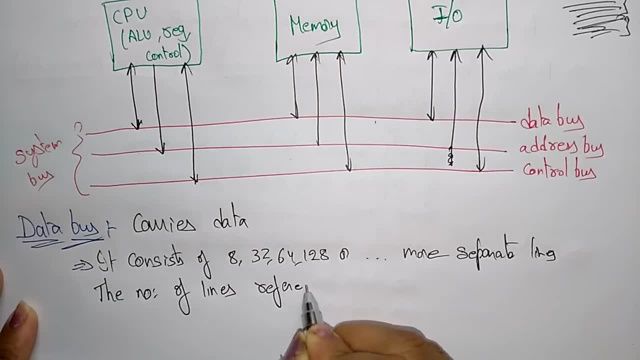 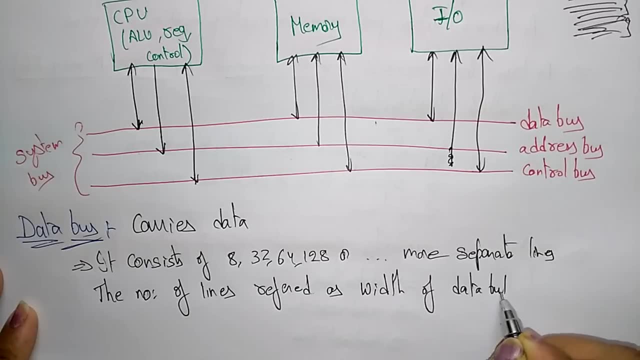 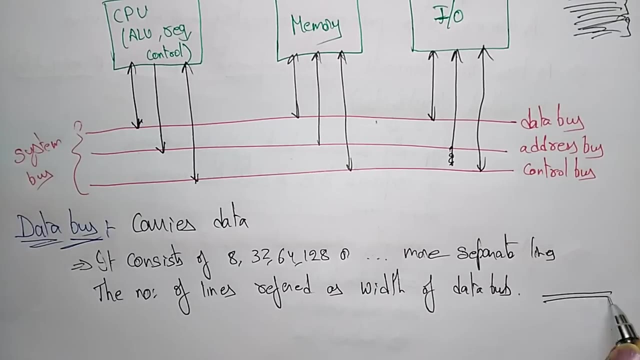 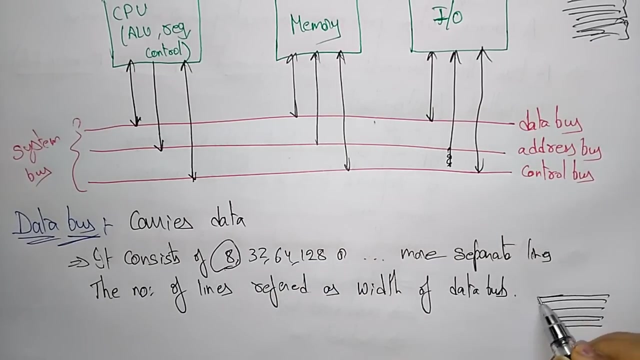 referred as a width of a data bus. width of data bus. so here each line carries only one bit. so you have to remember that. suppose the data bus is consisting of eight lines, suppose it is an eight bit means eight lines will be there in data bus. so each line carries one bit. each line carries one. 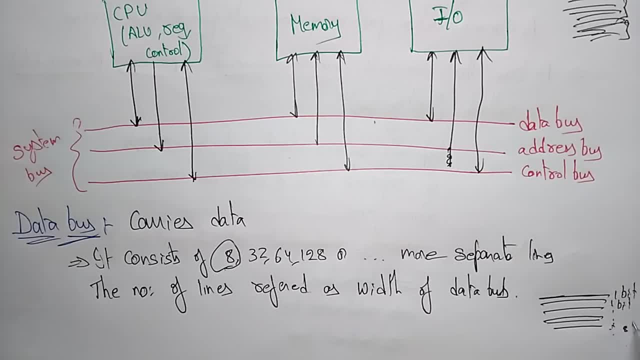 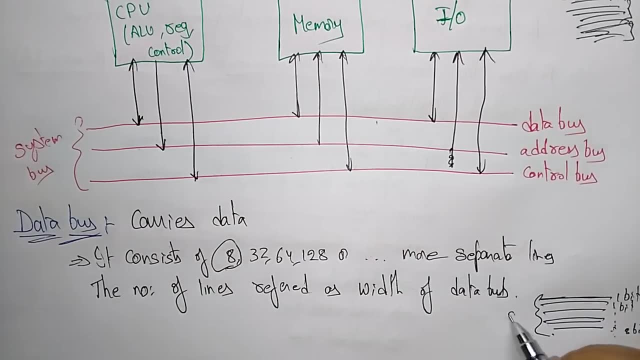 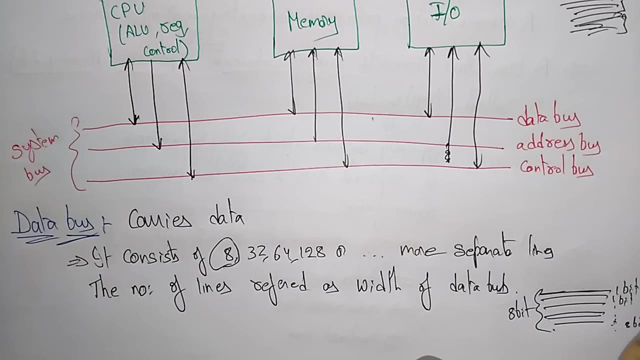 bit up to eight bits, okay. so the number of lines referred to as a width of a data bus. so the width of data bus here is eight bit means one byte. the width of data bus is one byte, sorry, two bytes. so one byte is equal to four bits. so two bytes, okay. so this is about the data bus. now let us see what is. 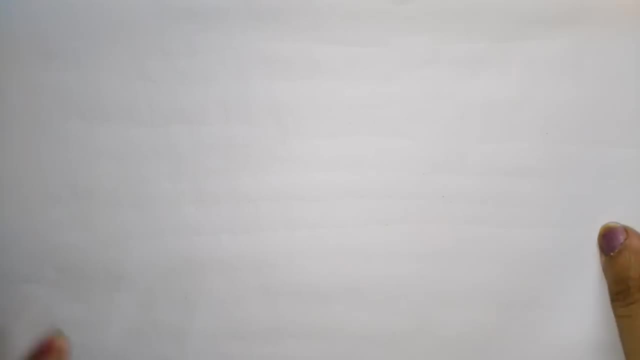 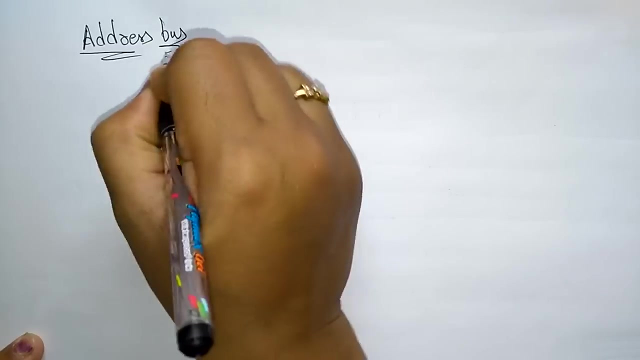 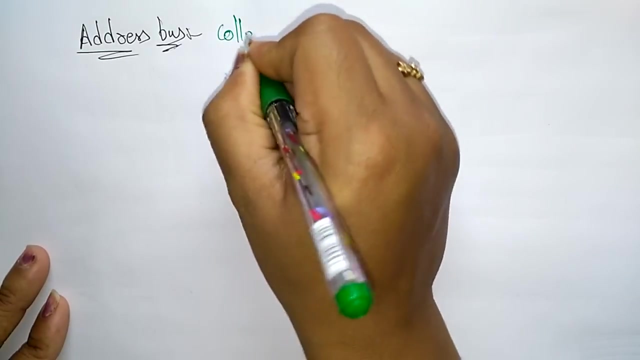 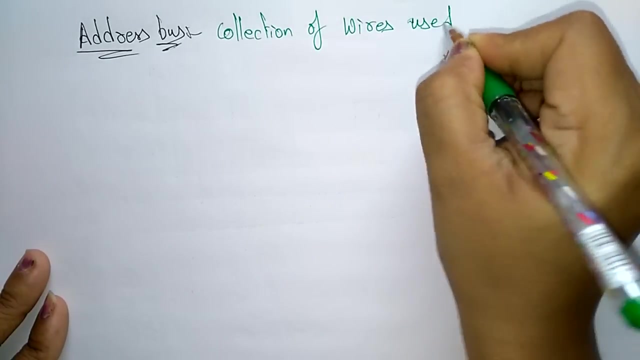 address bus. let me explain about the address bus. so data bus is used to carry the data. then what about the address bus? what is the use of the address bus? so address bus is nothing but it have. it is having the collection of wires, just like data bus. those wires used to identify 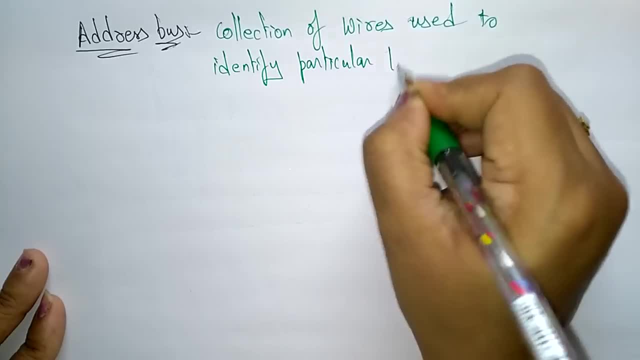 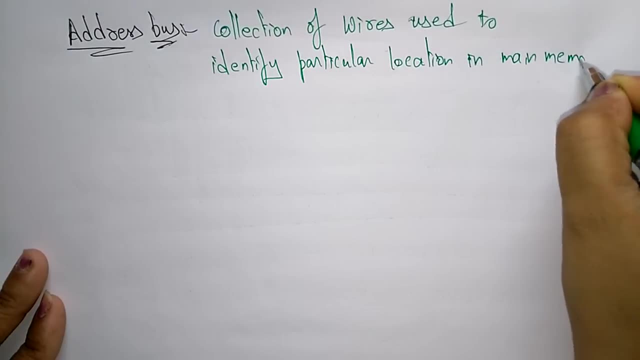 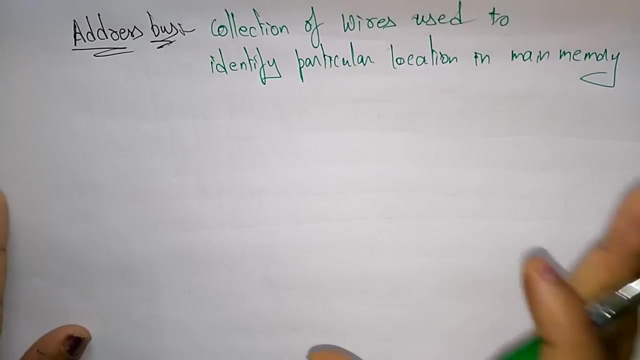 particular location in memory. so it is used to identify particular location in main memory. this is called address bus. so that is why the previous diagram i had seen that the address buses are you need and only one direction will be there, because that direction indicates to identify a. 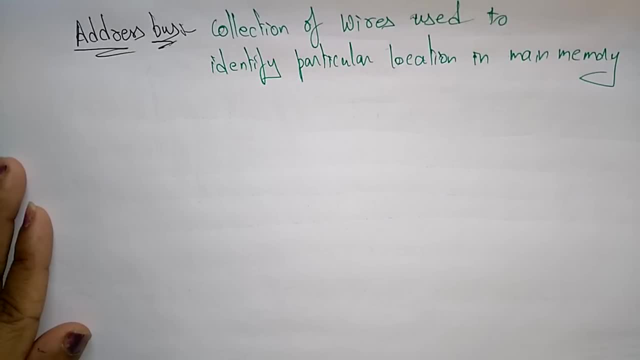 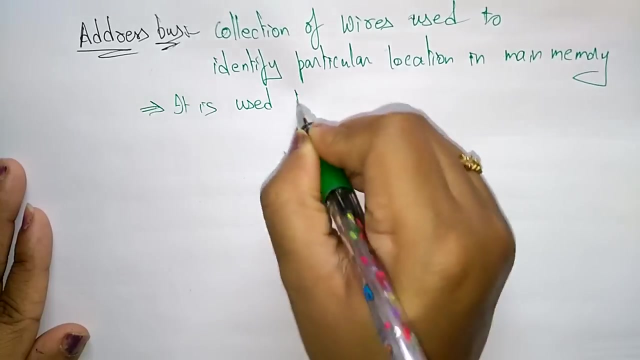 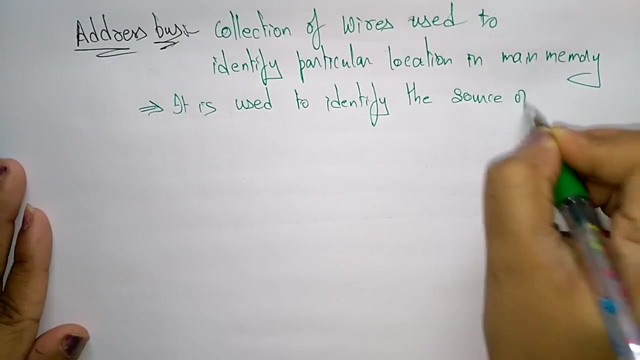 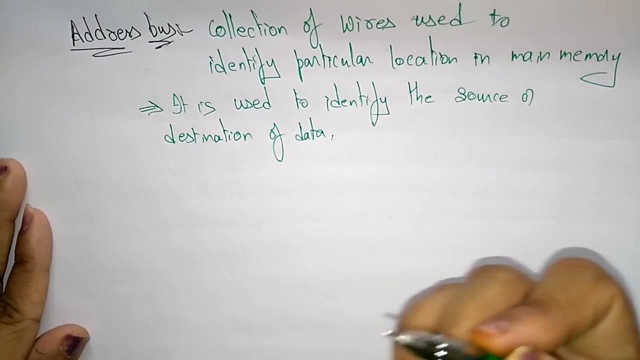 particular location in memory. so pointing towards to the memory means you identified a particular location in memory by the cpu, so it is used to identify the source for memory, source or destination of a data. The main use of address bus is used to identify the source or destination of data. Okay, so here example: the CPU needs to read an instruction or 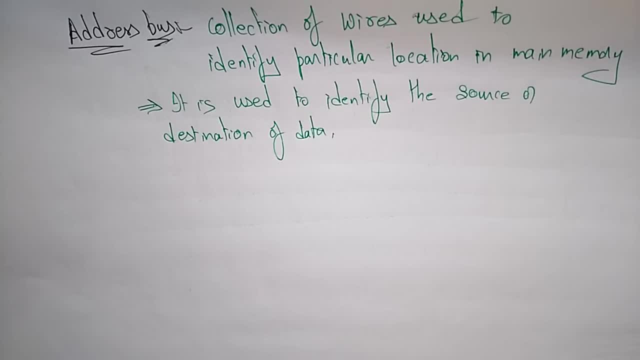 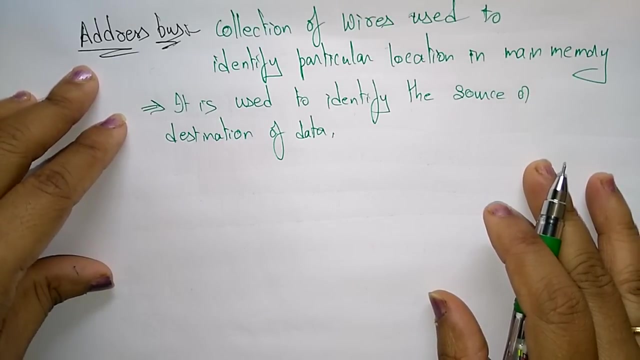 data from a given location in memory, just like the CPU wants to read a data from memory. So if it wants to read a data from memory, first it has to know where the data is present. So that will tell by this address bus. The address bus holds the address of the data. 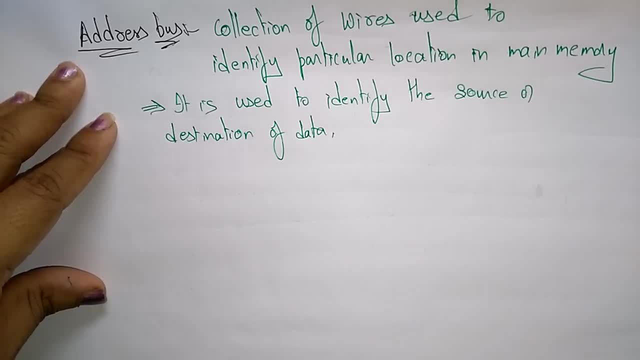 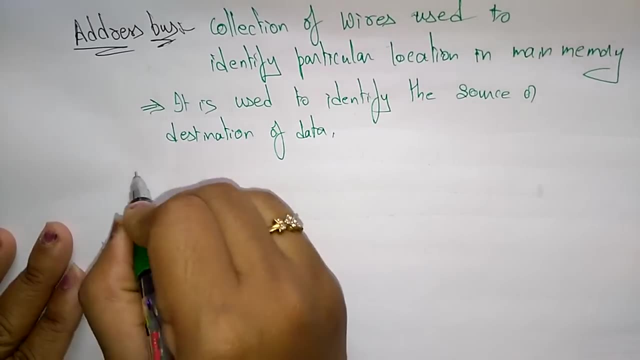 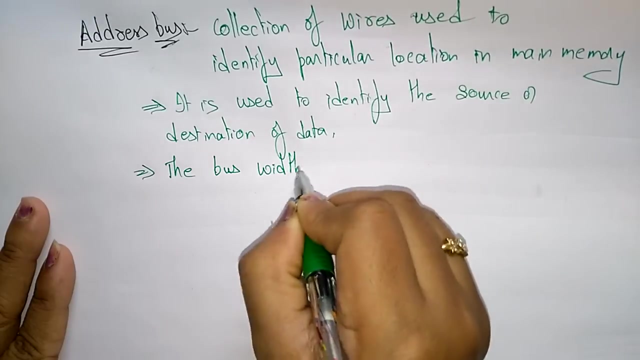 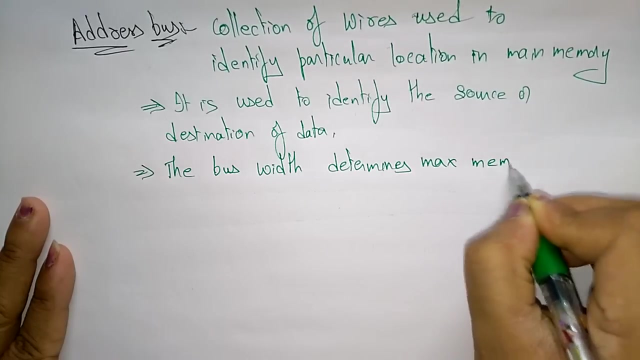 that data presence in the memory. So the CPU needs to read an instruction or a data from a given location in memory. And coming to the width of the bus, how can you say the bus width? the bus width, The bus width of address bus determines maximum memory capacity of a system. 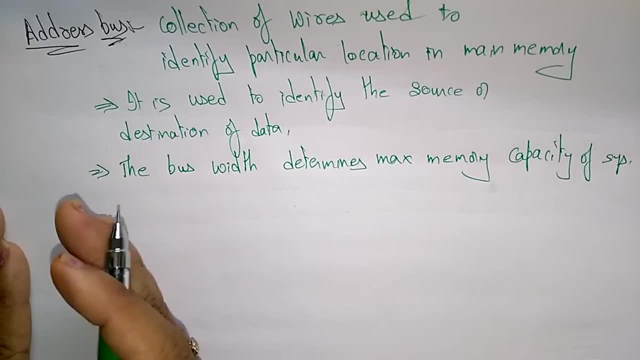 What it means. So the bus width of address bus, whereas data bus bus width is determined by the number of lines it referred carrying. Okay, so suppose 8 lines are carrying each line carries. So if 8 lines means the bus with this 8 bit, So how? what is address bus? because it 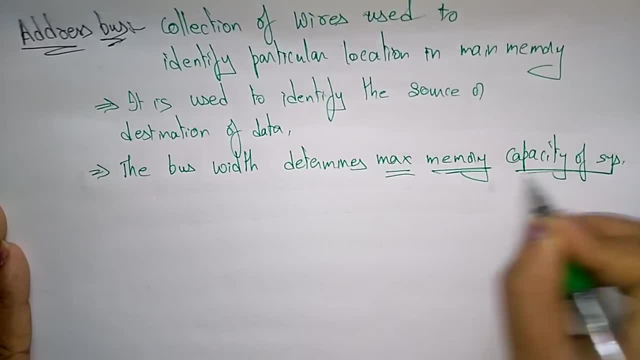 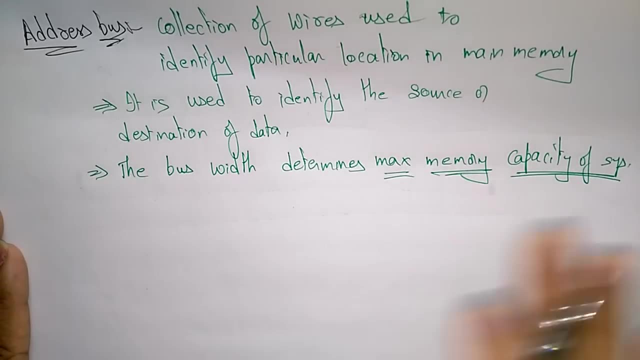 will be determined. it is determined by the maximum memory capacity of the system. So, whatever the procedure we are using, So that processor capacity, so the map memory capacity is depends upon this address bus determines the address bus. Let me explain the example. 8080 is a mic Stan micro processor cable. It determines the relative number of people call at will be 0. So if it automatically automatically store bus bus meaning 1.. 8080 is a micro origination configuration processing command. People just have to get the data taken by the user to detail the that data. but So that information is used to calculate the software price, number, YE, score, and I think that it would help a lot with the number of girls question. Let me explain. Let me explain with example. eight zero, eight zero is a big approach. my current life. 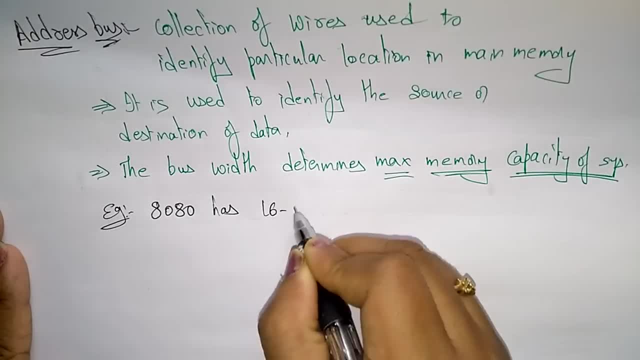 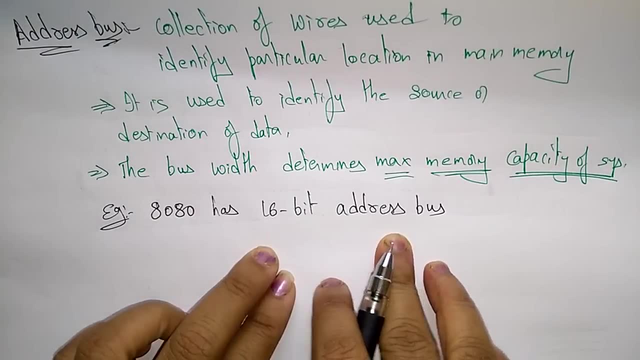 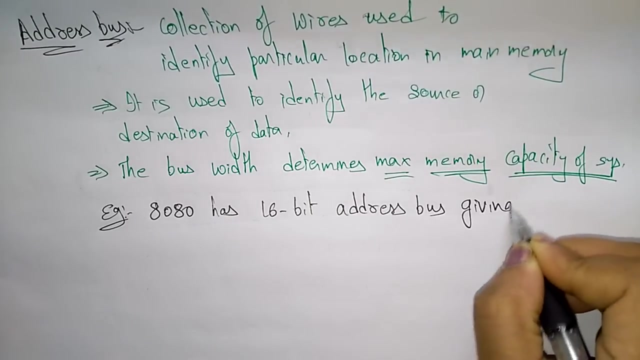 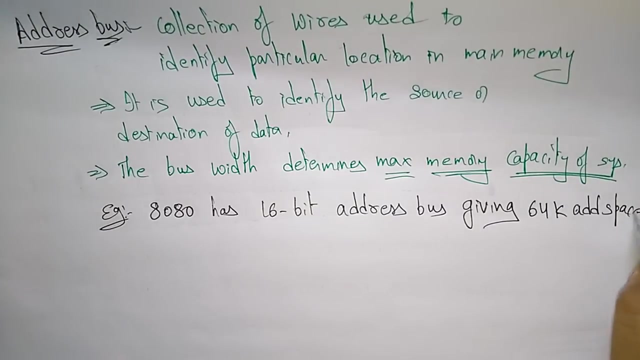 micro processor has, suppose it, it has a 16-bit address bus, means the address bus consisting of 16-bit lines, but it give 16-bit address bus giving 64 kilo address space. so even though it is a 16-bit address bus, it giving 64 kilo address. 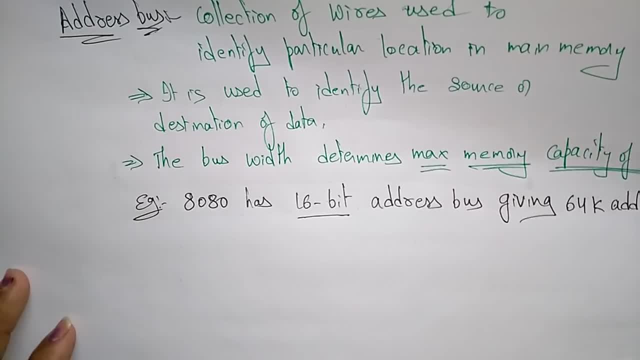 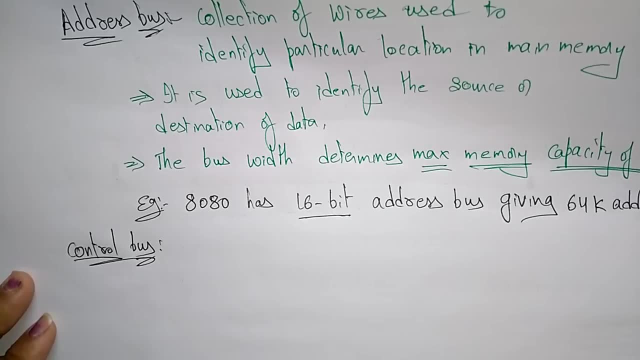 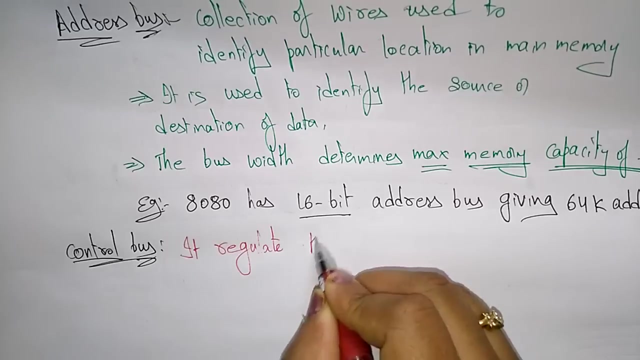 space. so that is about the address bus. now coming to the next, that is a control bus. so what is the use of control bus? control bus is nothing but it regulates. I already said, it always monitors all address and data bus, so it regulates the activity on bus. what it means: 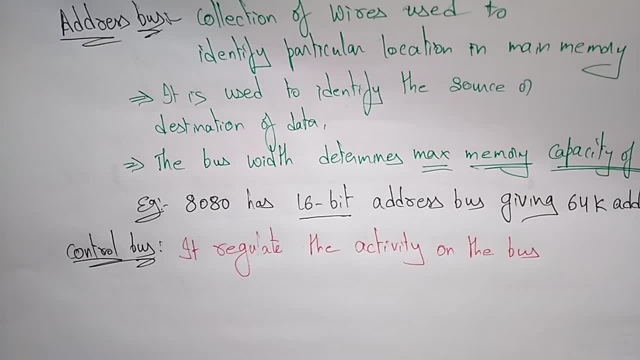 what it regulates the activity on the bus means it is saying when to read the data and when, when to put the data on data bus and when to read the address on address of the memory location. so, based on the address of the memory location, at what time the data? 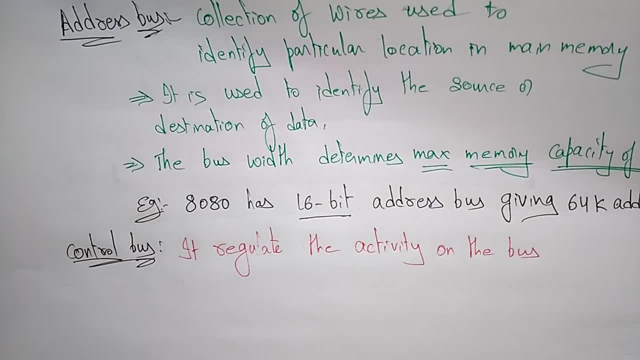 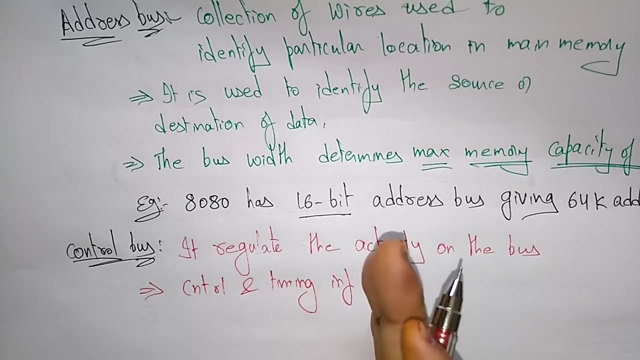 has to be put on the data bus, so, like that, it always regulates the activity on the bus, so it always controls and timing information. always control and timing information means it holds all the timing information related to the buses and it carries a signals that report the status of various devices. the 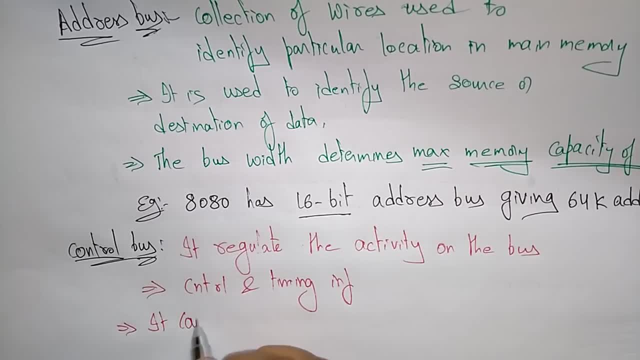 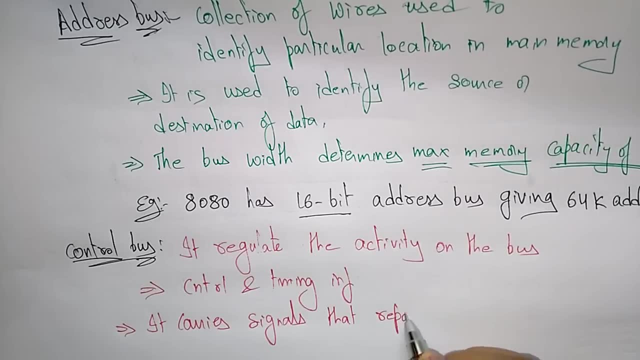 control bus holes or it carries signals that report that its signal is. report the status though various devices means whether radio it devices is looking at this. 뵈차요 juga. and that Понawar자uhu jingal hoon reض破 State pollen report. hut staff report. if they not pretending to find any data, Okيد 주세요. 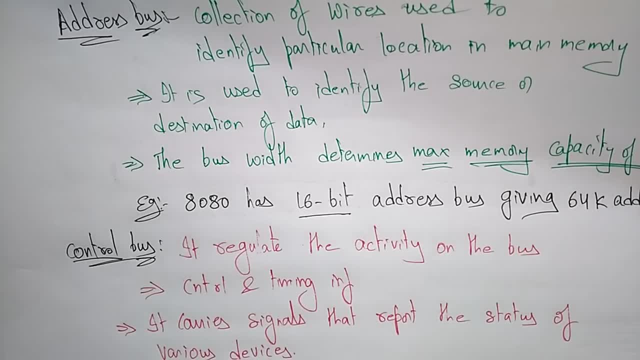 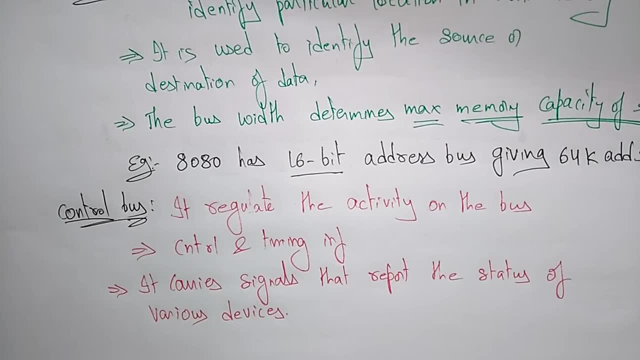 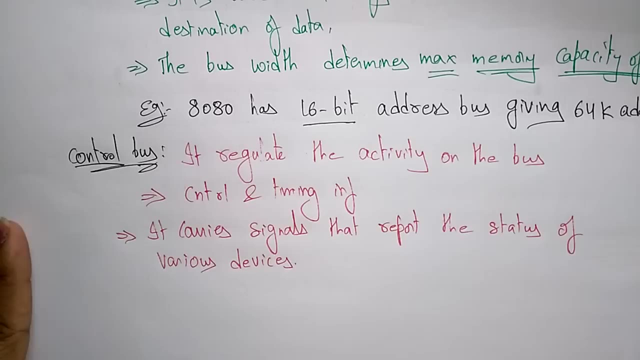 is ready or not, or is the device is sending any data like that. so it carries signals that report the status of various devices by this control bus. so there are different control signals will be there in the control bus. the control bus holds different control signals, like memory, memory read. 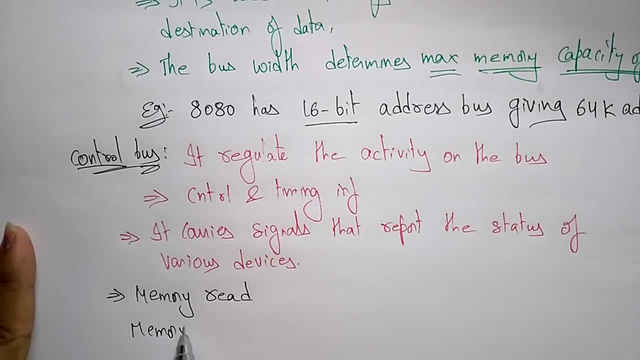 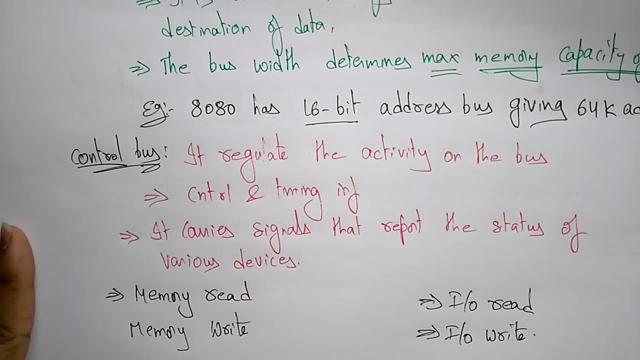 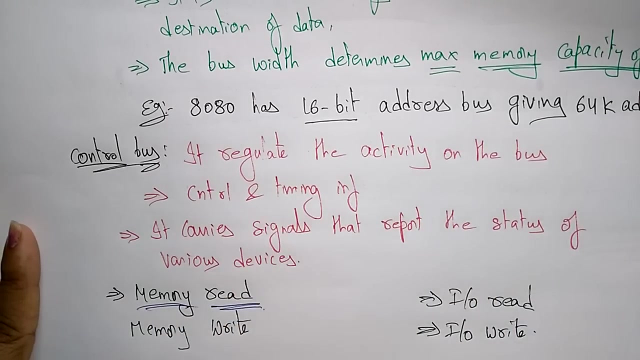 memory write, io read, io write, so like that. these are the different uh typical control signals hold by this control bus. so what this memory read means? so memory read nothing, but it causes data from address location to be placed on the data bus, so we have to get the date address location. 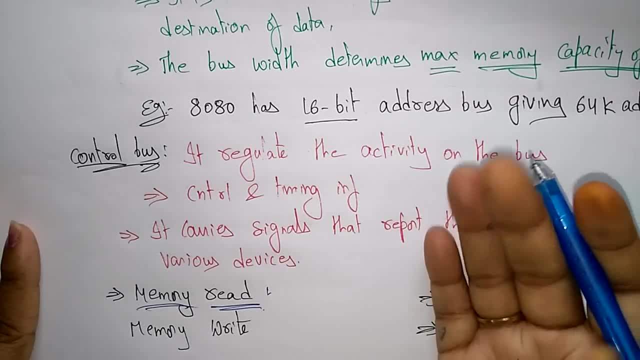 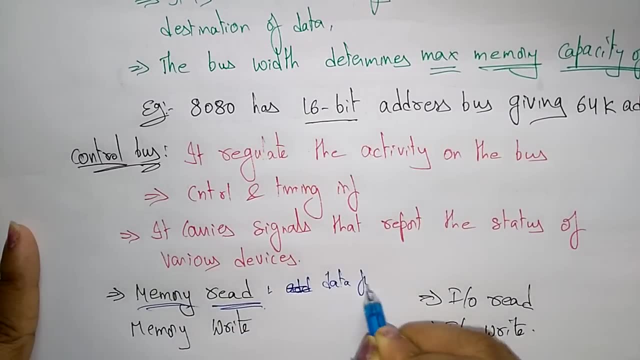 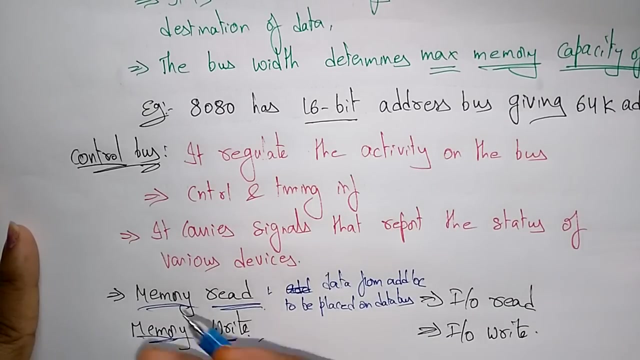 a data from address location to be placed on data bus. address should be the data from address location, right data from address location to be placed on data bus. so you just place the data on data bus with the help of memory read whereas memory write. the work of memory right signal is: 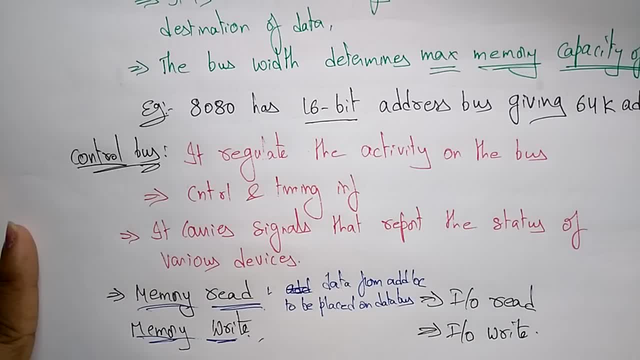 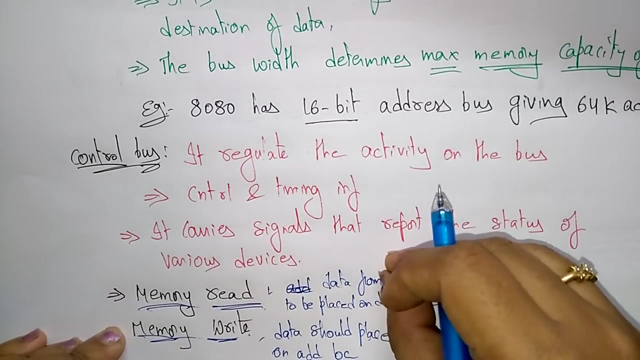 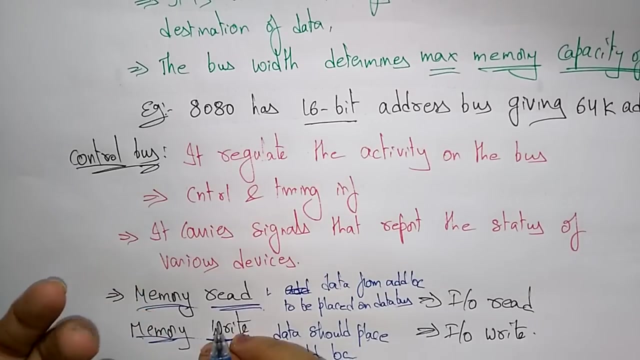 it causes data on the bus to write, written into address location. so means whatever the data that sends by the cpu, that data should be placed on the address location. data should place on address location. so from a particular address location means from memory, that data is placed on the data bus so that the processor can read the data, whereas memory write means whatever the cpu is. 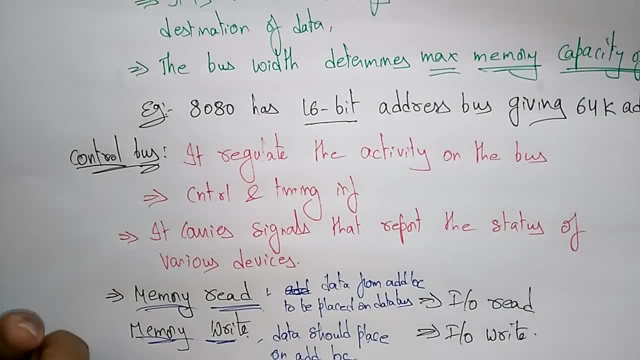 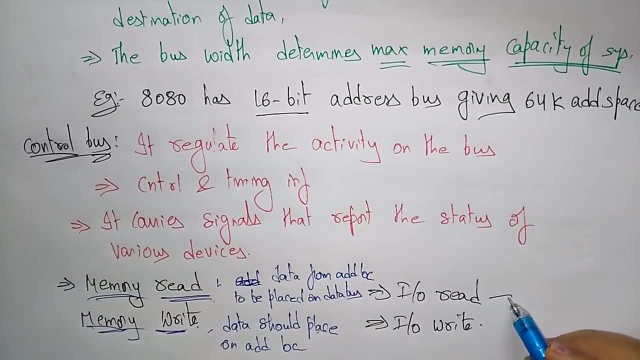 executed it, that should be placed written onto the memory. so that's why the data should placed on the address location of a memory. in the same way, i o read means data from address i o ports to be placed on the bus, whereas i o write is data on the bus to be output to the address of i o ports. so just memory. 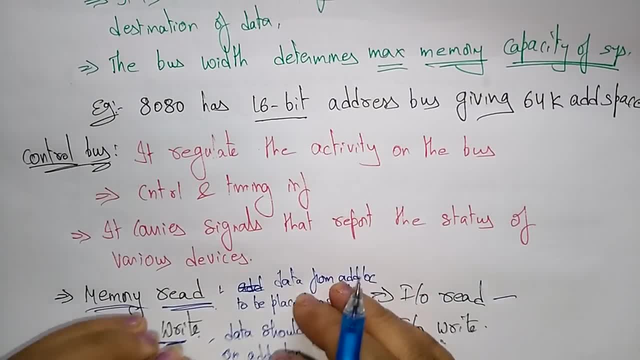 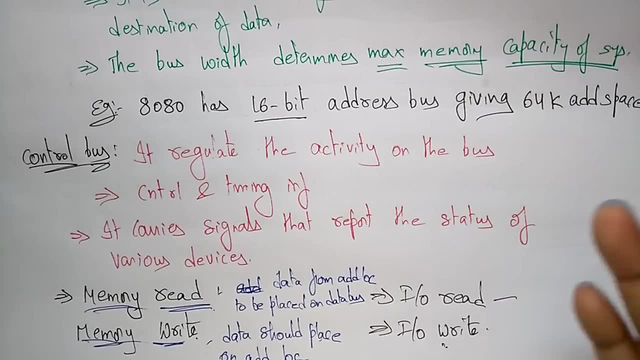 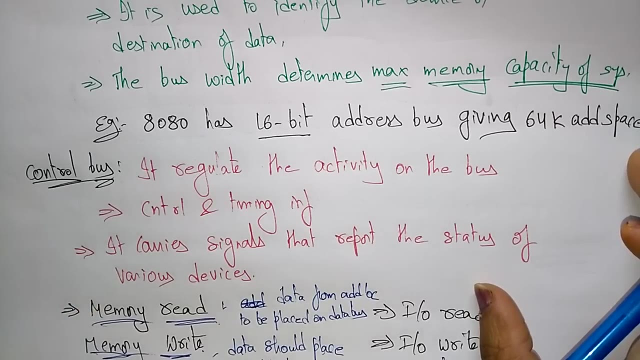 read, memory write. i o read, i o write, or the different signals. you call it as a control signals means it indicates the control bus. so what action you have to be do is you have to do a memory read means the bus has to read the memory read, or it has to do the. 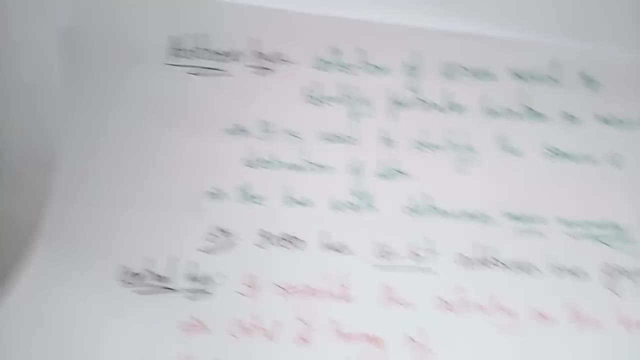 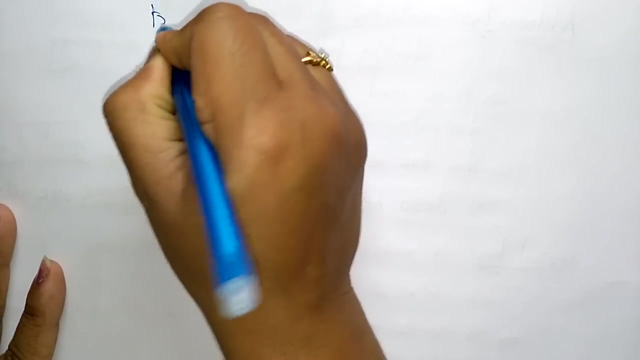 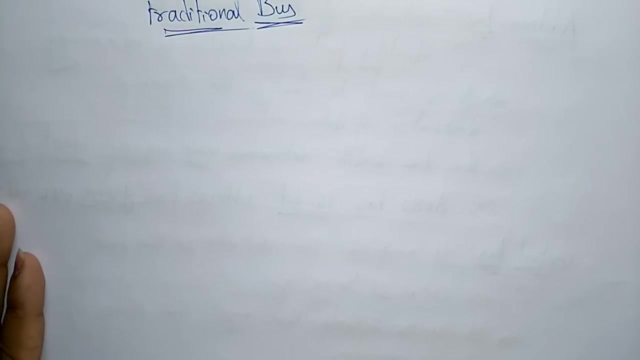 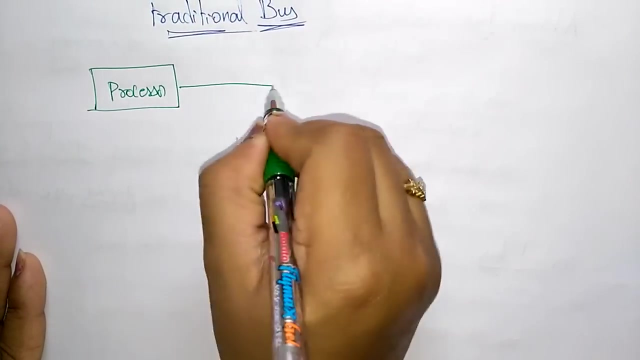 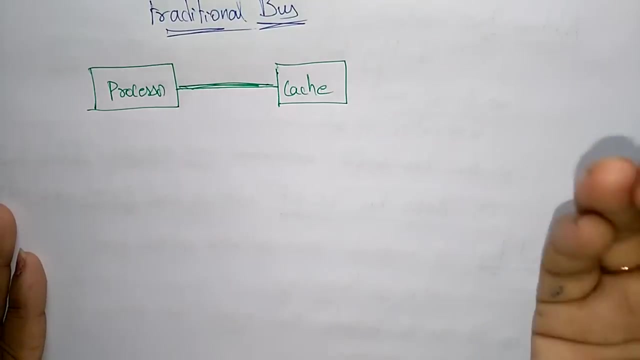 memory write operation, or i o read operation, or i o write operation, like that. so let me uh explain with some traditional bus architecture, a traditional bus. so here let me take this: a processor is there. a processor is connected with some local bus, with the cache. cache is a memory, it is a memory unit a. 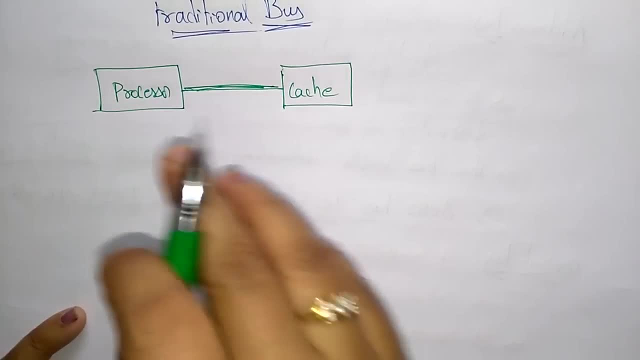 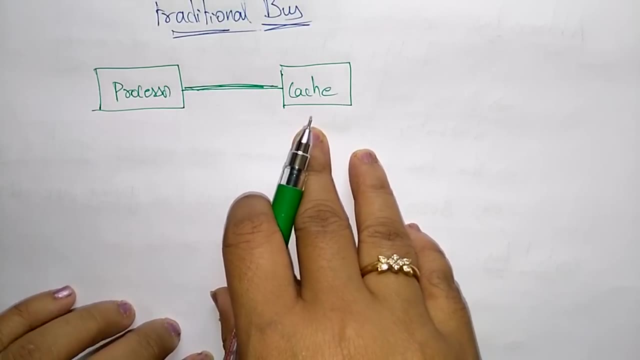 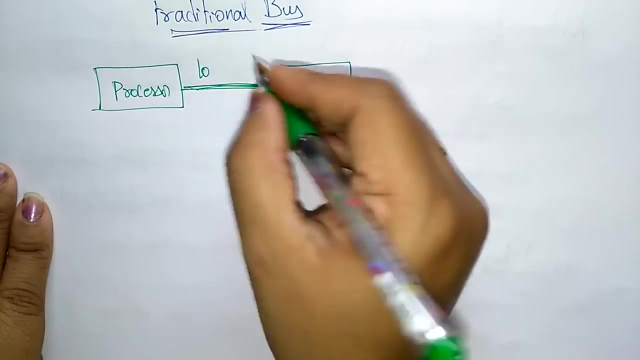 small memory unit that is present in the processor. okay, so whatever the data the processor want to be executed uh that, or want to send to the other devices, that data will be stored in the cache. cast is the fastest storage device after register, so this is a local bus connecting between the processor and cache by using the local. 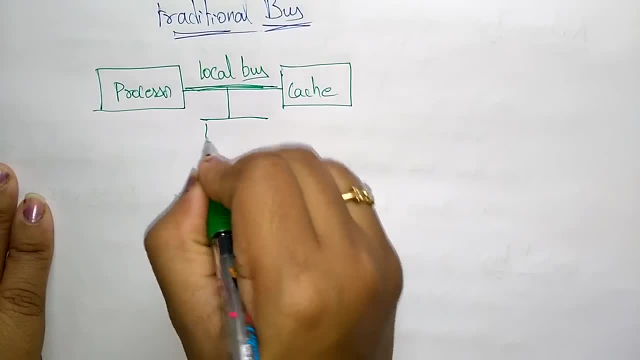 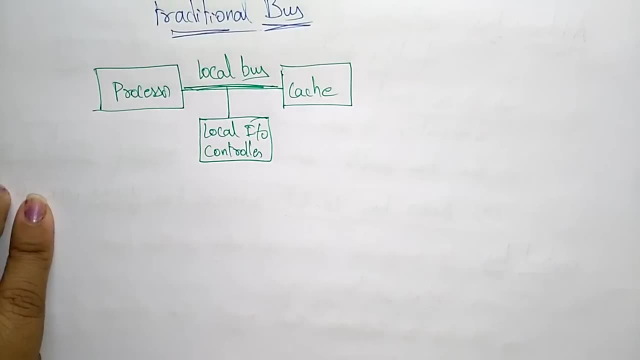 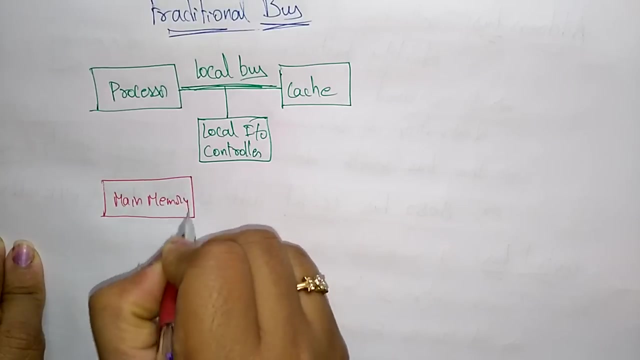 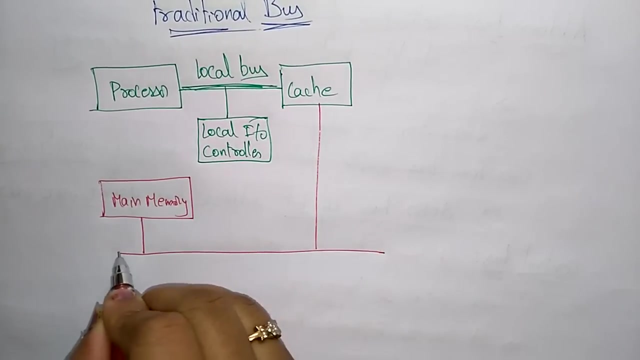 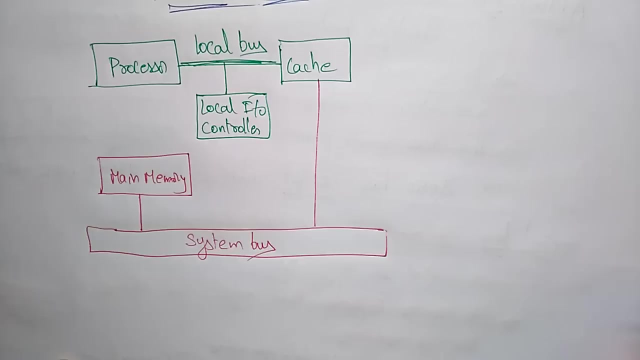 bus and here some local i o controller is there: input output controller. okay, now coming to the main memory. this is the main memory and this main memory and the cache are connected by using the system bus. here this is a system bus and after that, with the system bus, is connected with some expansion. 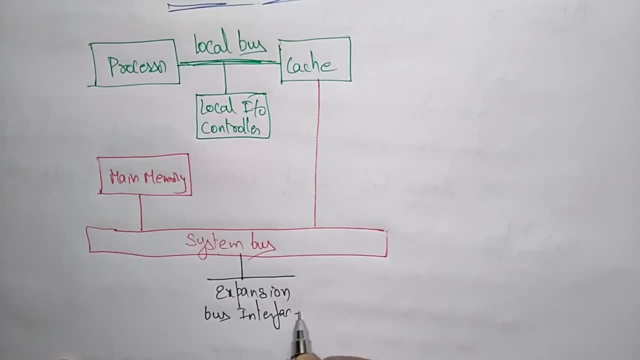 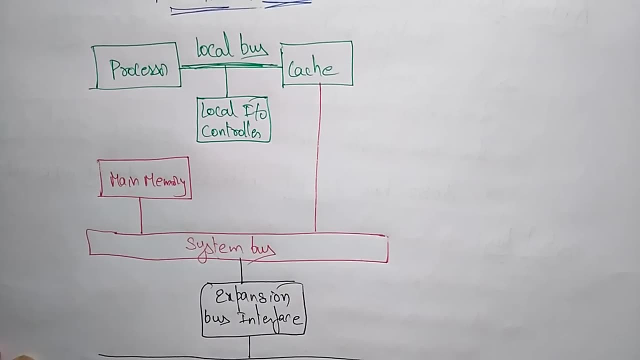 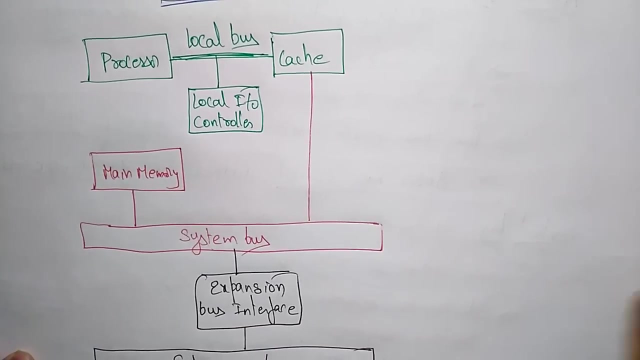 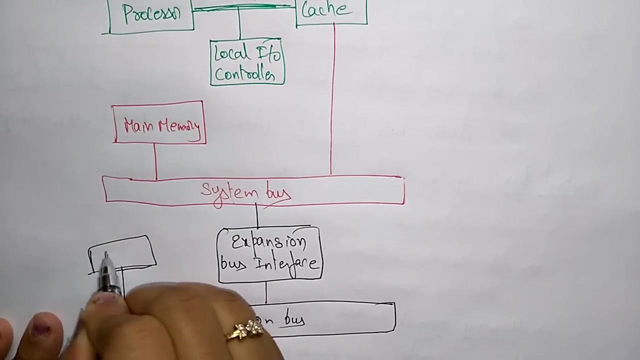 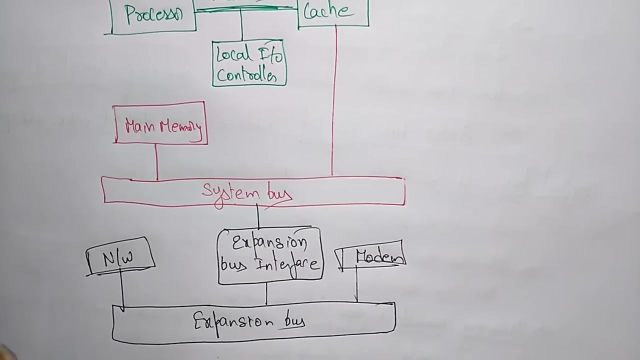 bus interface. okay, so here an expansion bus slot will be there, so not only the system bus, you can also connect an extra buses to your device, your system, whenever it requires. if you need, you can connect some expansion slots. so here a network unit will be connected, or some modem is connected, or some serial, some input output devices will be connected. 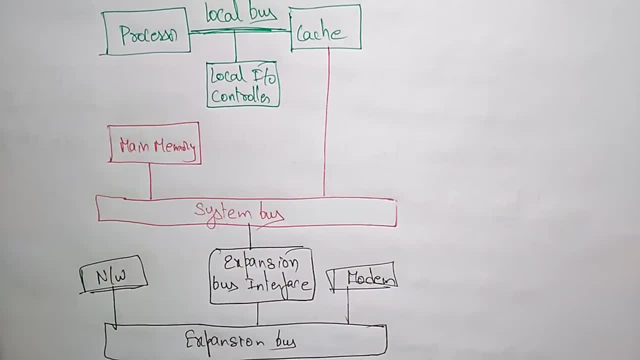 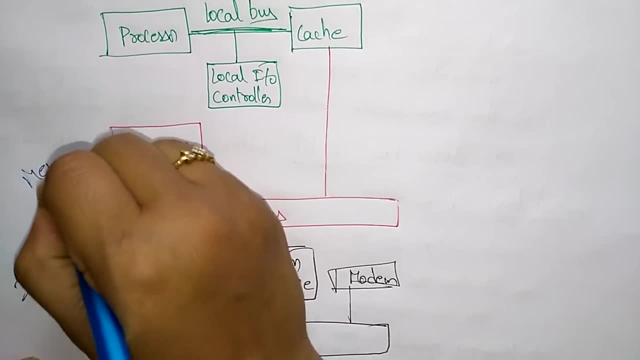 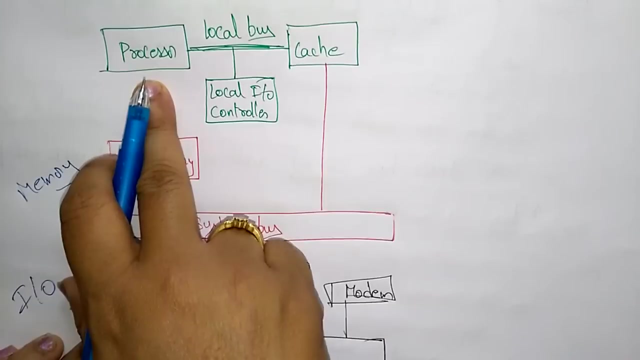 now let us see. what is this? a traditional bus. so here, the one thing you are, whatever the devices that are- these are the input output devices or the memory devices- is not directly connected to the processor. okay, so whatever the processor is doing, that first sends to the cache. so the cache is connected to the system bus.